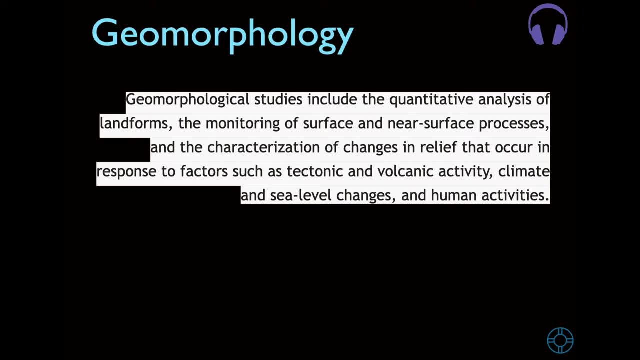 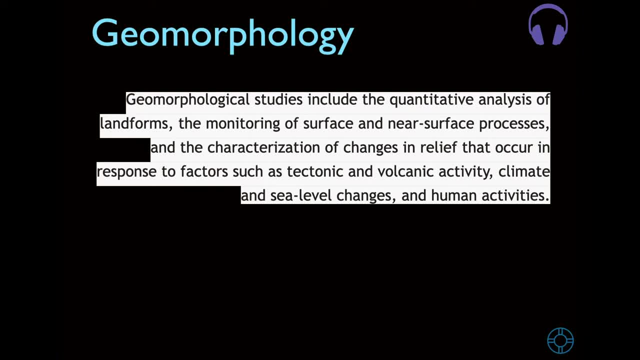 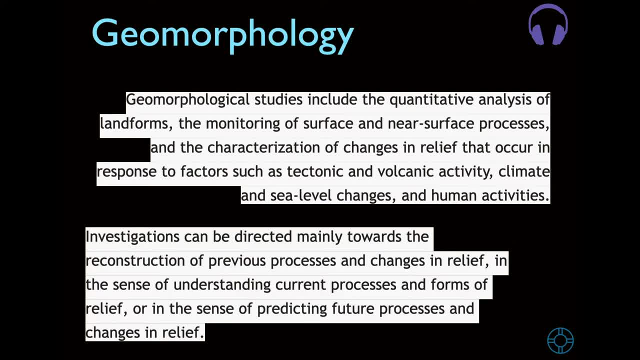 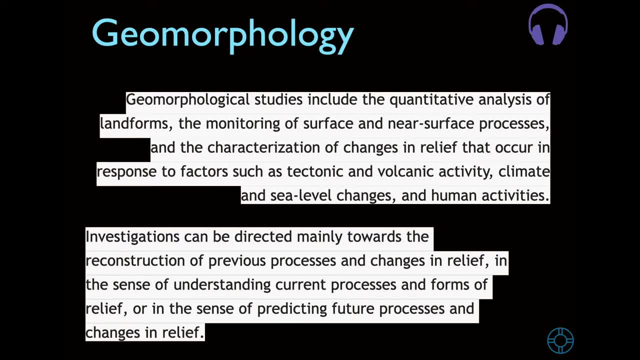 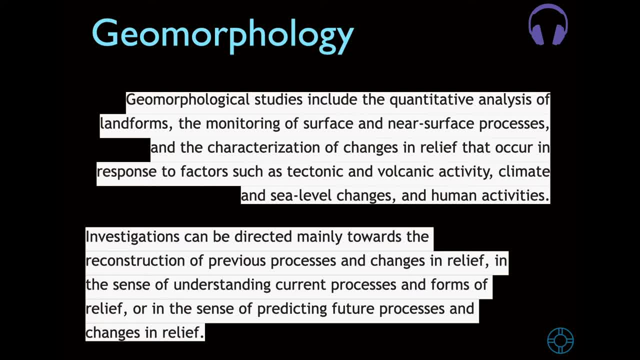 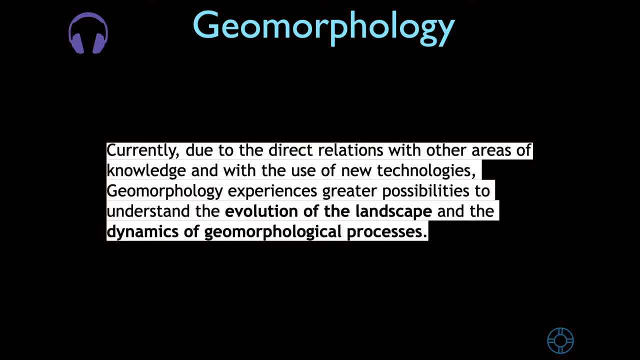 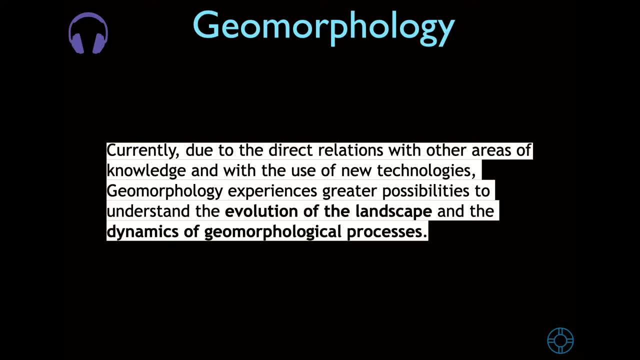 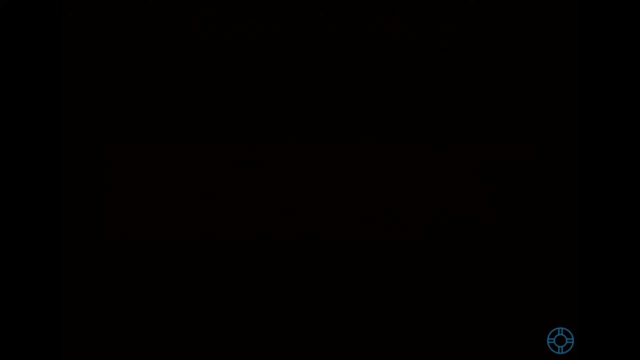 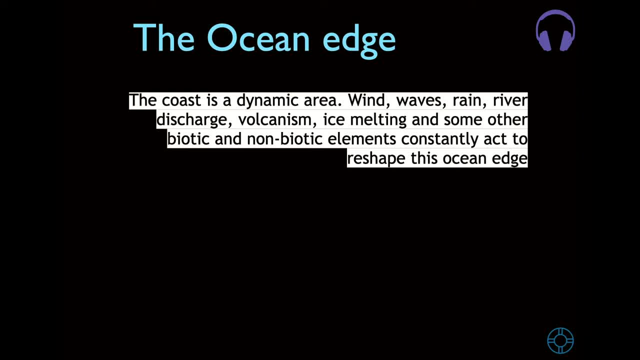 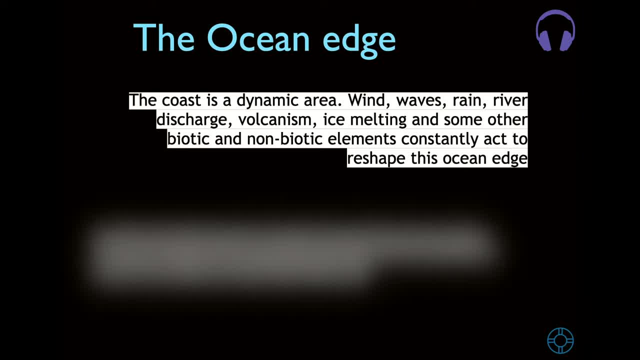 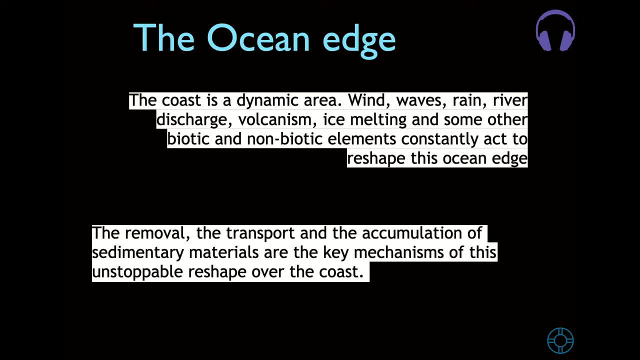 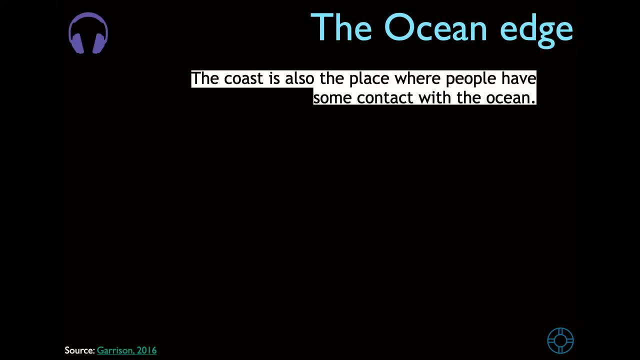 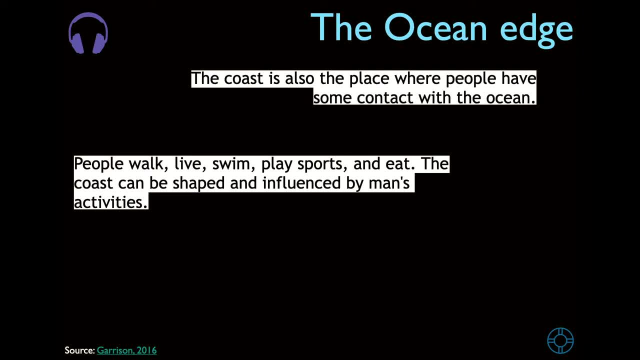 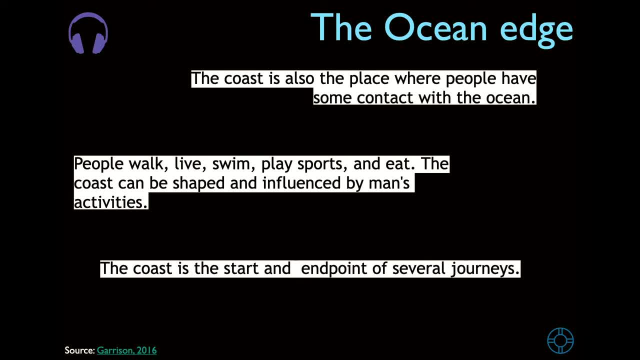 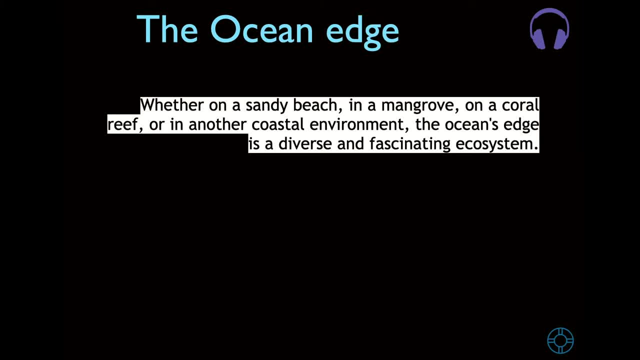 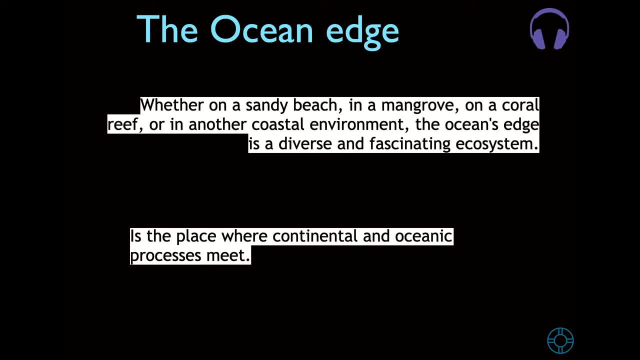 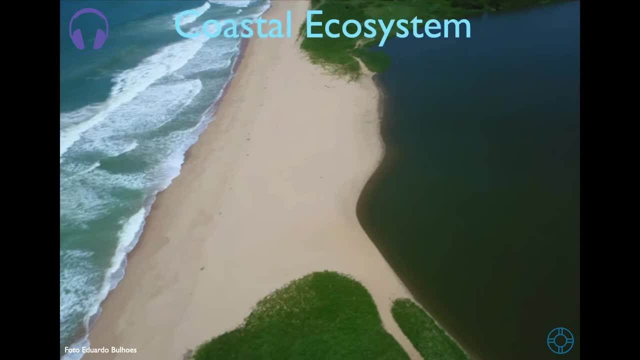 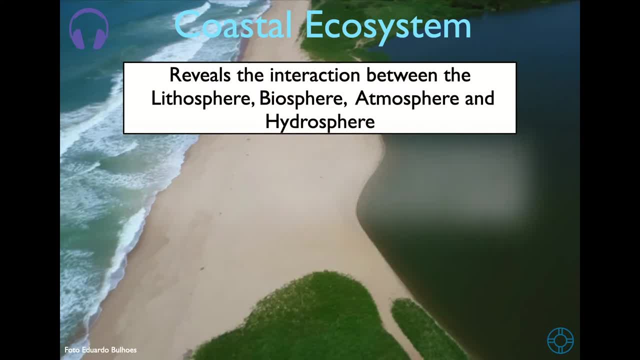 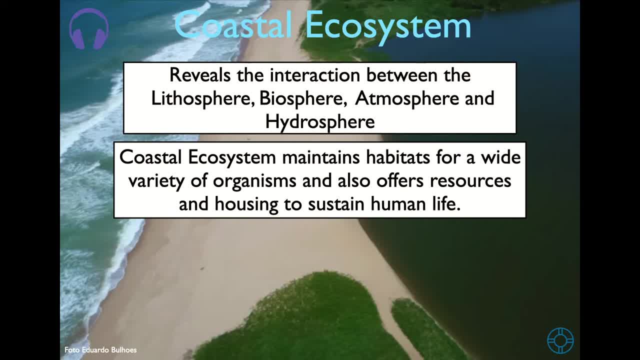 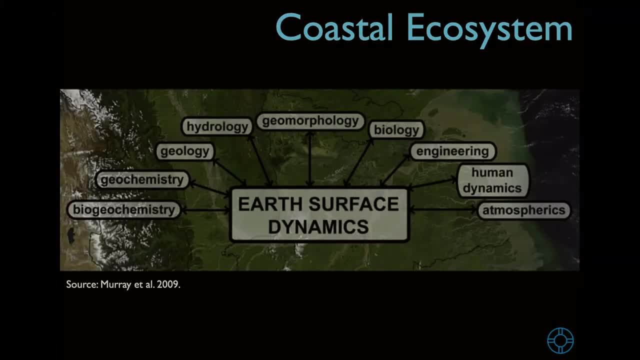 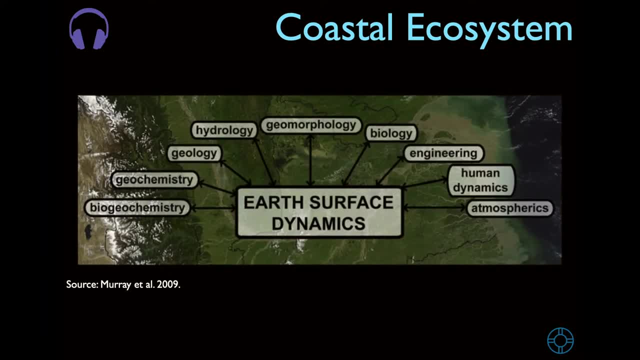 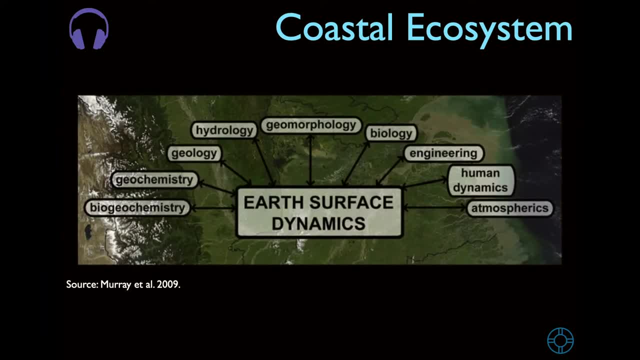 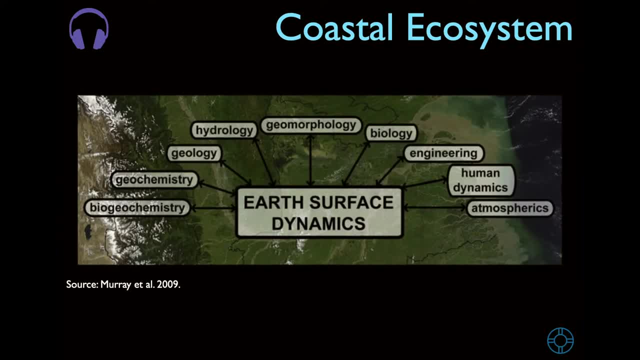 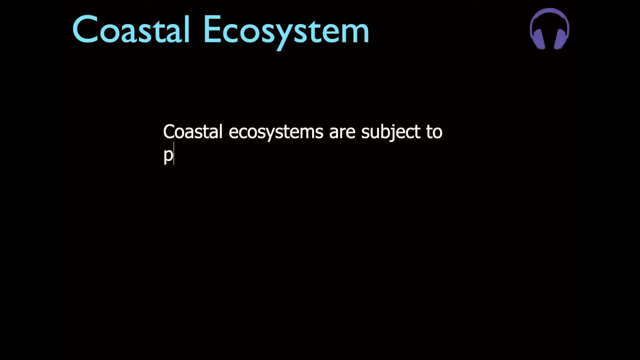 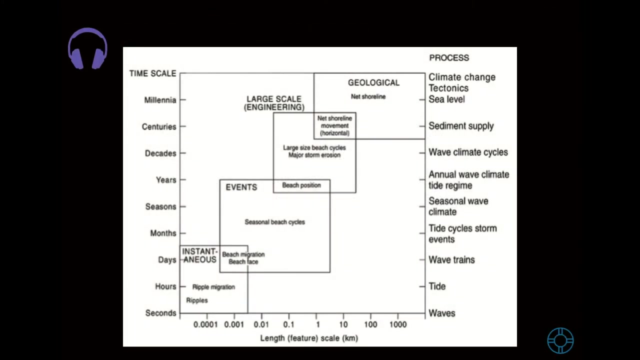 Coastal ecosystems are subject to physical forcing through a whole suite of environmental variables operating over multiple space and time scales. Let's see what is next. This is a very important graph. It shows the relationship between coastal sedimentary feature scale and their temporal variability, together with the four major time-space paradigms used. 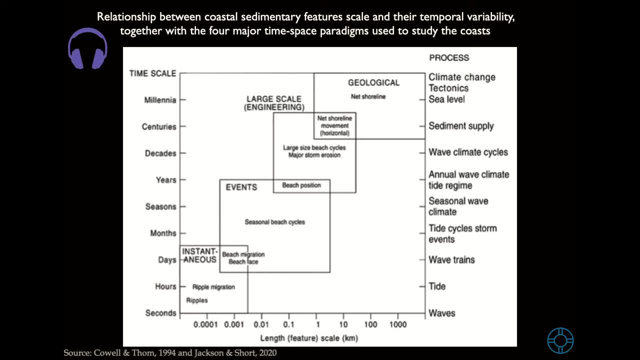 to study the coasts. Coasts are one of the most dynamic environments on Earth and one of the most responsive, much visible with the naked eye. As most coastal studies focus on a component of the system, example, a sandy beach or an estuary, usually over a. 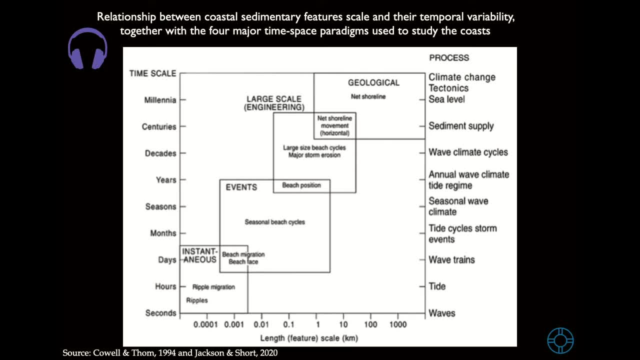 limited time frame. they must adopt the appropriate length and time scales to both observe the process and the bad responses and the negative consequences. In this graph, the y-axis on the right presents the scale of processes ranging from waves up to climate change. This axis includes, from the bottom, the tides. 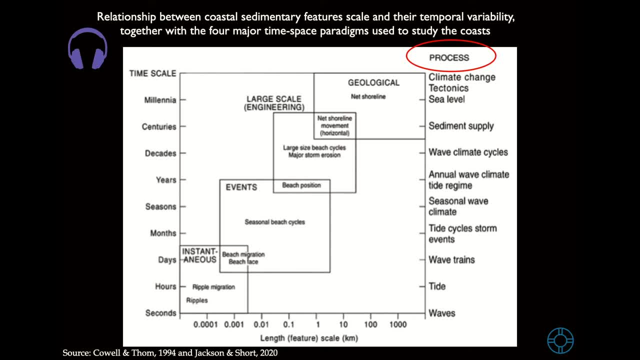 the wave trains, the tidal cycles and storm events, the seasonal wave climate, the annual wave climate and the tide regime, the cycles of wave climate, the sediment supply, the sea level and tectonics. Those processes are related to multiple time scales that can be seen in the left y-axis, The time scale in which 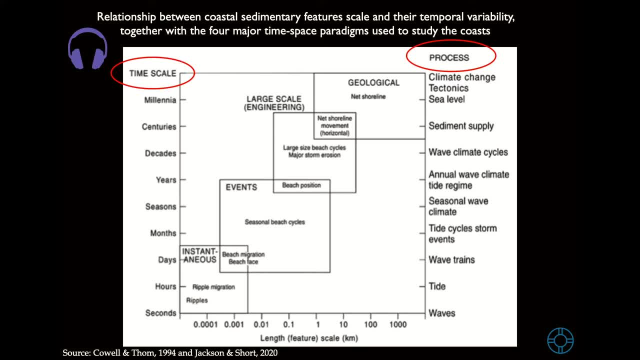 the processes occur varies. for a second time. The more time scales it has, the more time period to the millennial time scale. It also includes from the bottom, the scale of hours, days, months, seasons, years, decades, centuries and etc. At the 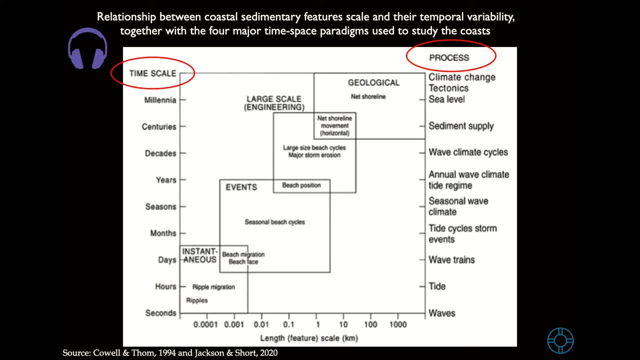 X-axis we can see the spatial scale which includes the length of our inter-restless features. They range from the left- considering the millimeter scale- up to the right, where is a thousand kilometers scale? Inside the graph there are four major time space paradigms used to study the coasts. 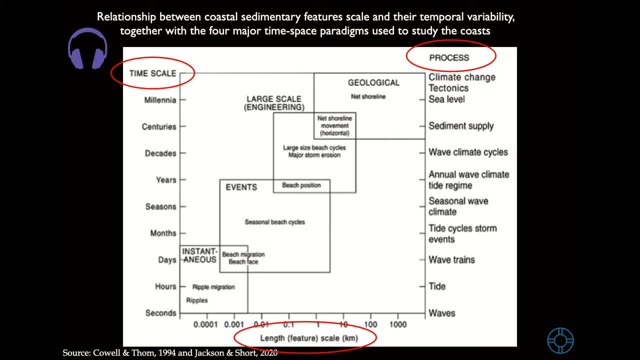 From the bottom. we consider the instantaneous scale, where ripples and ripples migration and modification rely on the time scale of seconds to days and are restricted to small spatial scales reacting to waves and tidal processes, Then the event time space scale is, in this one, the investigations about seasonal beach. 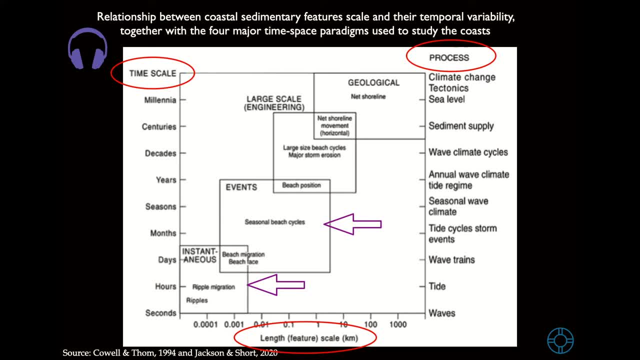 cycles are taking monthly to annual time scales, considering some regional spatial scale, and reacts to seasonal wave climate processes. The next one is the engineering large scale, where investigations range from years to decades and maybe centuries time scales regarding processes that include sediment supply and long-term wave climate cycles. Those investigations also 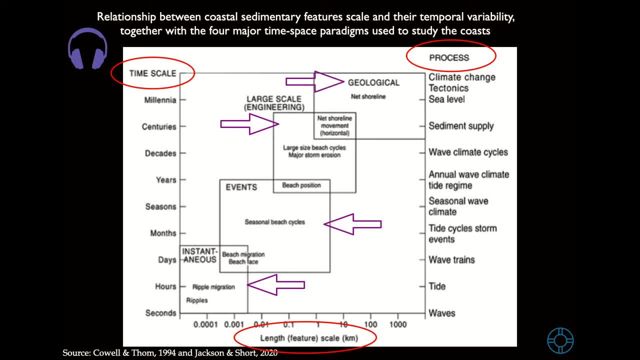 deal with larger spatial scales. Finally, the geological time space scale deals with processes that occur from centuries to millennial time scales. Then we add the climate change space scale, which is based on spatial time scales from various antescapes and focuses on climate change, tectonics and sea level oscillations- processes at a spatial time scales of 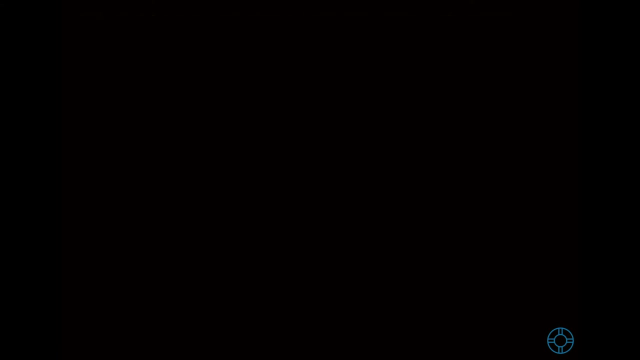 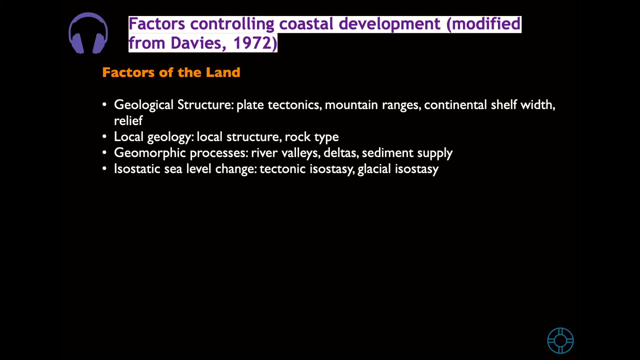 hundreds to thousands of kilometers. These are some factors controlling coastal development, modified for more, Modified from Davis 1972,. there are some factors from the land and we can talk about geological structure, like plate tectonics, mountain range, continental shelf width. 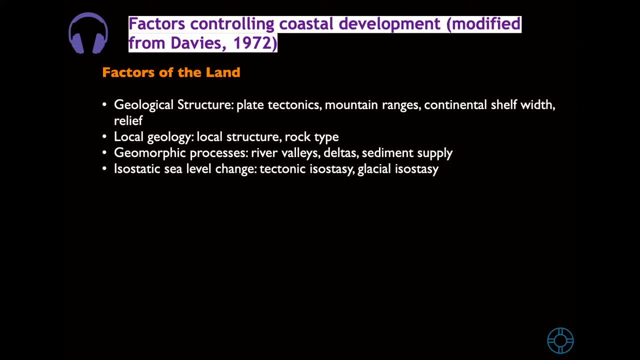 and relief. We can talk about local geology, like local structure, rock types. We can talk about geomorphic processes like river valleys, delta, sediment supply and isostatic sea level change, tectonic exostasy, glacial exostasy. 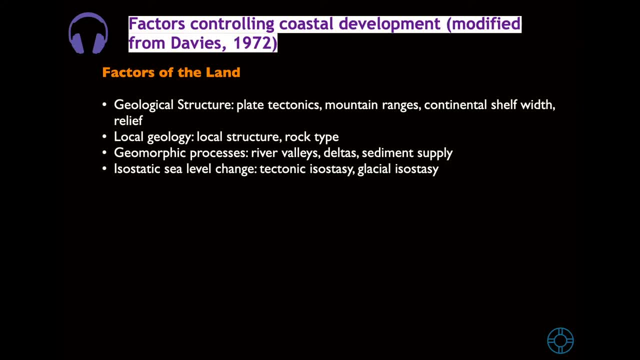 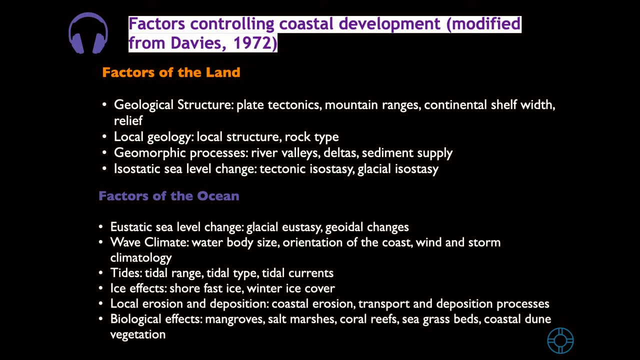 And there are also factors of the ocean controlling coastal development, And these are ecostatic, sea level change, like glacial exostasy, geoidal changes, wave climate, water body size, orientation of the coast, Wind and storm. climatology can talk about tides, tidal range, tidal type, tidal currents. 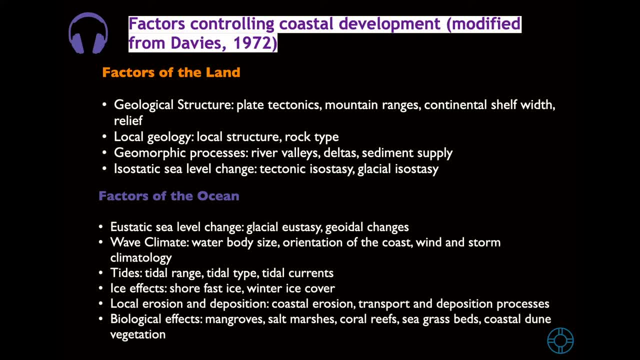 We can talk also about ice effects: shore fast ice, winter ice cover. also local erosion and deposition, coastal erosion, transport and deposition process and biological effects. the presence of mangroves, salt marshes, coral reefs, seagrass beds, coastal dune vegetation. 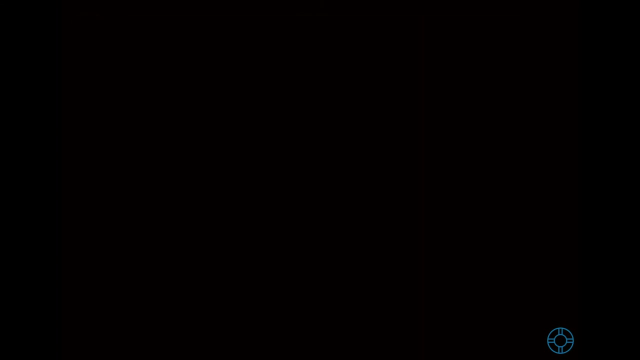 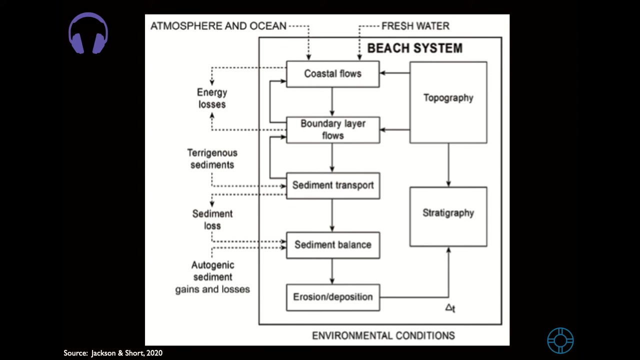 etc. This graph is also extremely important. It presents the morphodynamic relationships between boundary conditions like topography, inputs from the atmosphere and the sea. This graph is also extremely important. It presents the morphodynamic relationships between boundary conditions like topography. 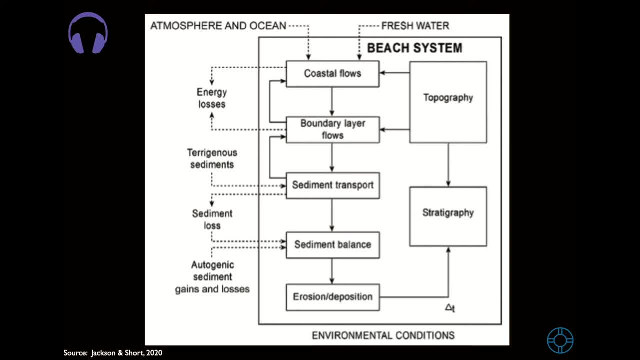 inputs from the atmosphere, from the ocean, the regionals and autogenic sediments and interactions like those in the central boxes, including coastal flows, boundary layers, sediment transport, sediment balance, erosion and deposition, And the resulting surface morphology. again, the topography and underlying stratigraphy. 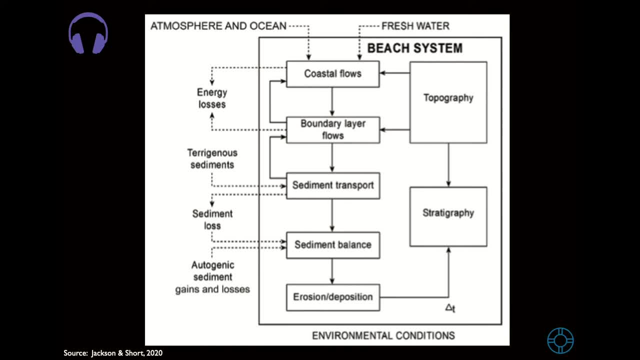 in the coastal environment. This is the core of landform morphodynamics. We must be aware of both the interrelationship between the bad response morphology to processes dynamics, and the ensuring positive and negative feedbacks between the two as they work towards an equilibrium relationship. 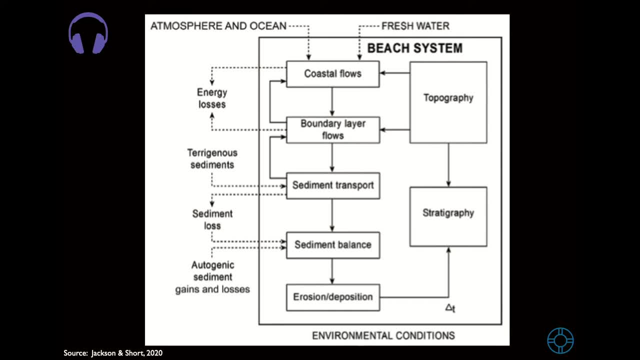 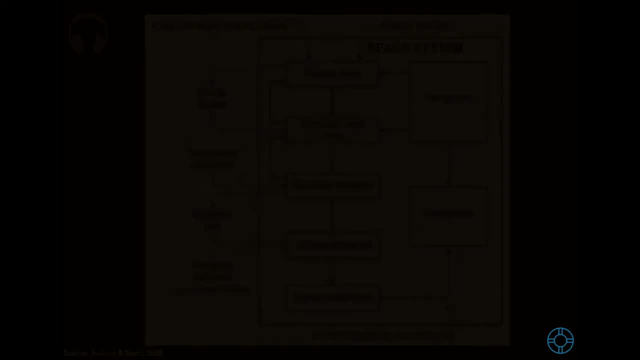 DER PRINCIPLE. So all this includes the作 math You learn touch and webinar. in the measurements That equilibrium is rarely achieved, hence driving changes. This map from Wiles & Spencer 1995 shows the global tectonic condition of the coast. 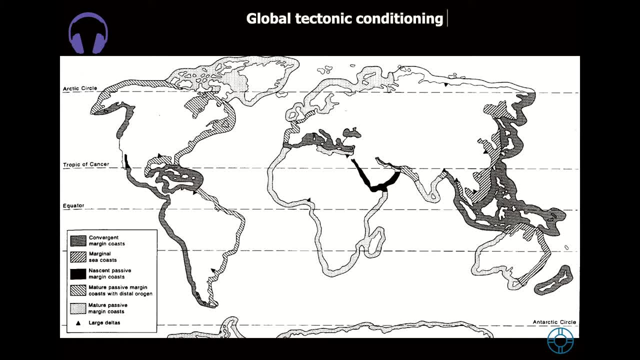 As you can see, it is a matte tilage which correlates with how the 친구 quando sexo share, there was a species, or the species single with a trotzdem body. This trulyuso that equilibrium. The breaking down of the air then realizes the cut, as if we realize that equilibrium. 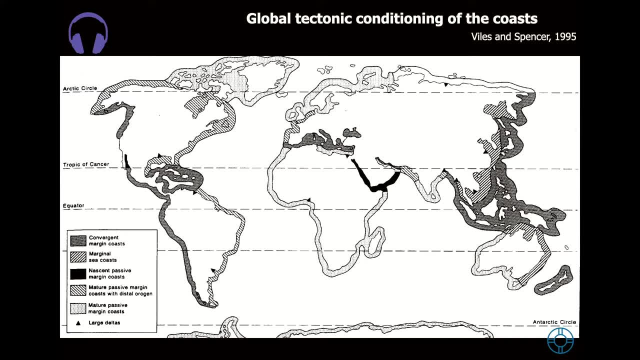 is rarely achieved, Hence driving changes, The dependent changing of the coast: South America, Africa and continental China. the coasts are quite different from its global tectonic origins. In South America we have the eastern part. where is Brazil? we have this matured, passive margin coast with distal origin. 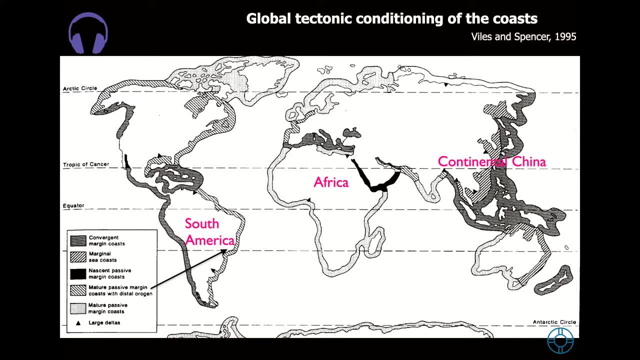 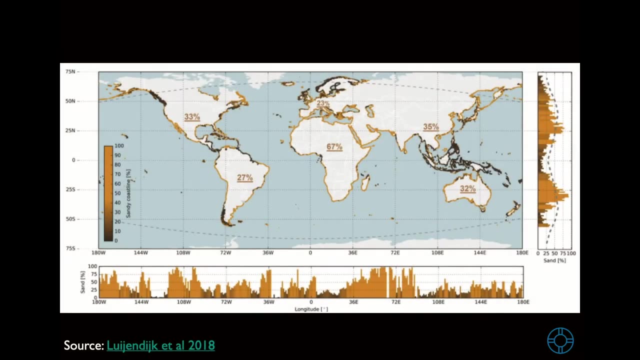 In the West we have converged margin coasts, Africa presents major passive margin coasts, And continental China presents marginal sea coasts. We are going to talk about this later. This map and these graphs are also very important. This shows the global distribution of sandy coasts and was constructed by Luzendik and 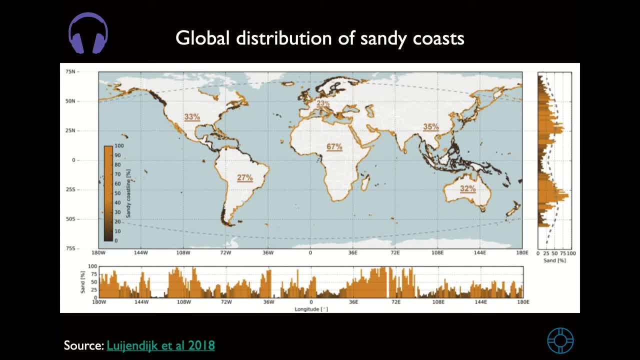 his collaborators in 2018.. The colored dots along the world shoreline represent the local percentages of sandy shorelines. Yellow is sand. dark brown is non-sand. The subplot to the right presents sandy shorelines. The lower subplot represents the relative occurrence by degree of latitude, where the 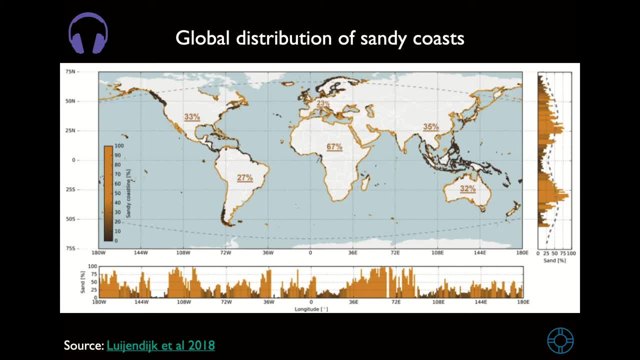 dashed line shows the latitudinal distribution of sandy shorelines reported by previous studies. The lower subplot represents the relative occurrence of sandy shorelines per degree of longitude. The curved dashed gray lines in the main plot represents the ice-free shoreline. The blue dashed gray lines indicate the percentage of sandy shorelines averaged. 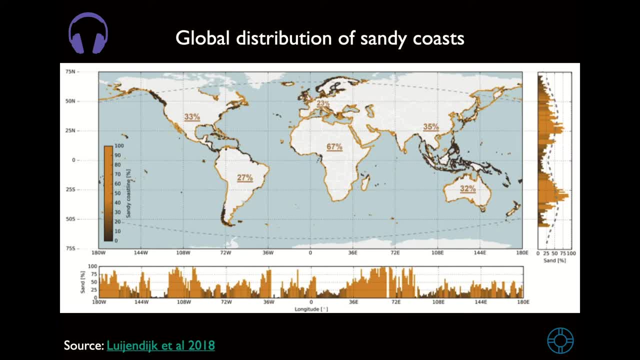 per continent. The analysis showed that 31% of the ice-free world shoreline is sandy. The continent with the highest presence of sandy beaches is Africa- 67%, While in Europe only 23% of the shoreline is sandy. Asia is sandy in 35% of its coasts. 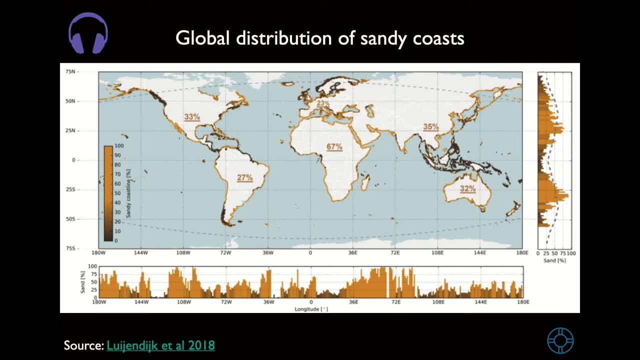 and Oceania is 32%, North America 33% and South America 27%. The global latitudinal distribution of sandy shorelines shows the relative occurrence of sandy shorelines per degree of latitude. shows a distinct relation with latitude and climate. No relation is found with longitude. 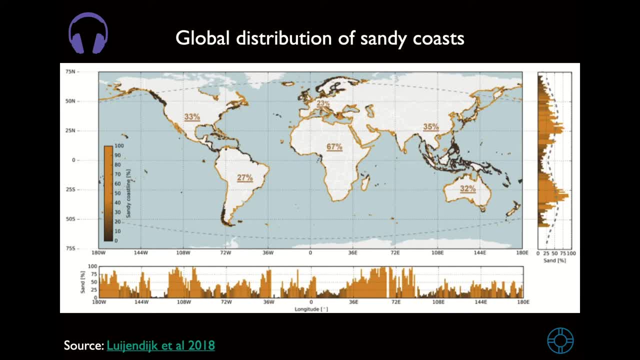 The relative occurrence of sandy shorelines increases in the subtropics and lower mid-latitudes, with maxima around the latitudes near 30°S and 25°N. In contrast, the urds are relatively less common in the humid tropics, where mud and mangroves are most. 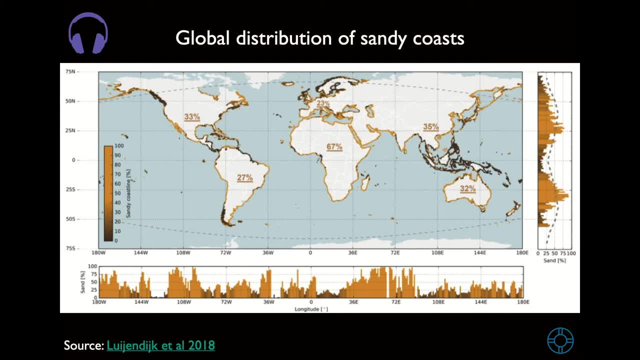 abundant. due to high temperatures and rainfall, The percentage of sandy shorelines decreases beyond 50%. parallel. This latitudinal distribution of sandy shorelines is in line with the latitudinal variation of the common sediments. In this particular case, the force distribution of sandy shorelines is 80% and the participation 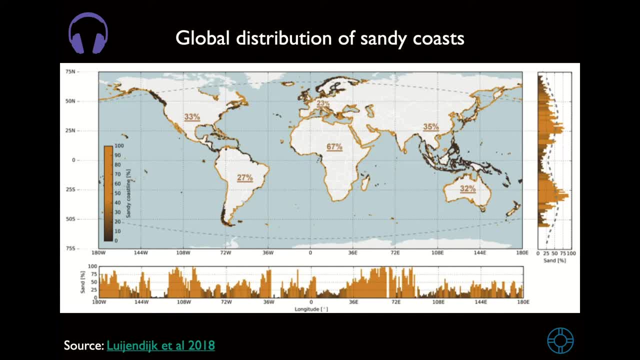 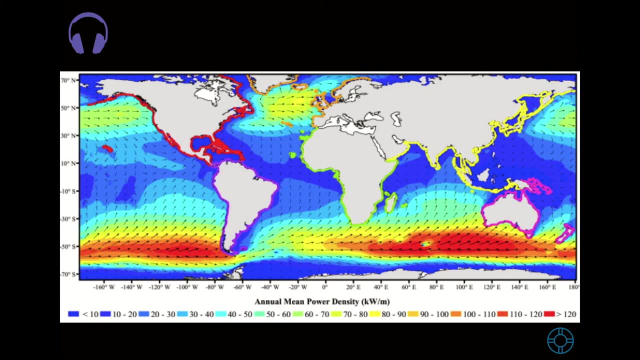 inner continental shelf, also reported by previous studies. This map, built by Gunn and William 2012,, shows the global wave environment, and colors represent the annual mean power density of waves along the global ocean and we can identify areas of major energy and minor energy along the global ocean. 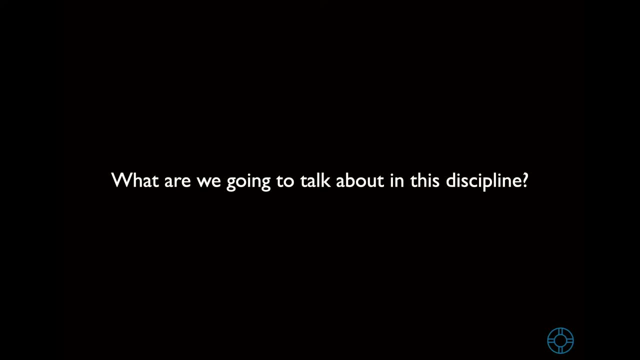 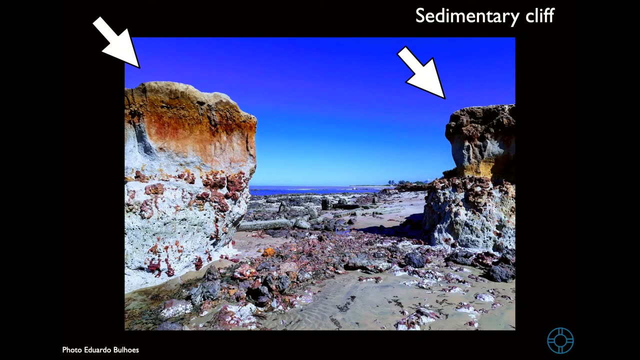 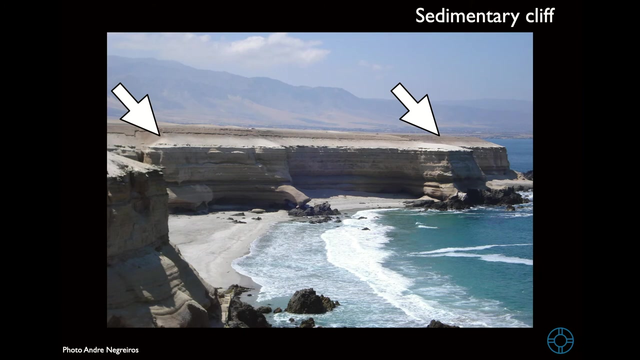 The Cenozoic Hemisphere is our world view of the earth and is dedicated to the impact on the global life. This map shows the continental surface of the European Union and the continental surface of the Atlantic Ocean. The Cenozoic Hemisphere is a map showing the global Arctic climate with itsheads. 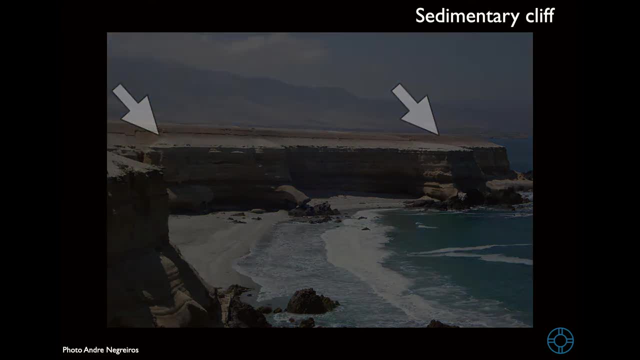 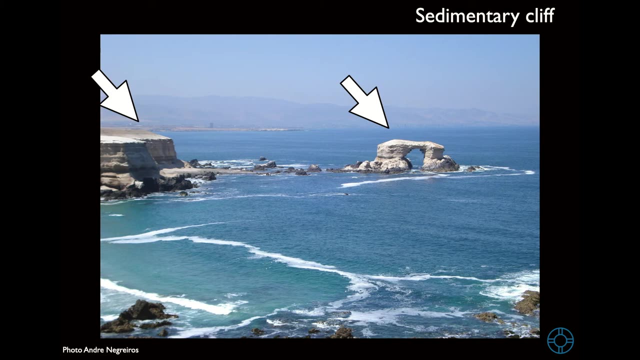 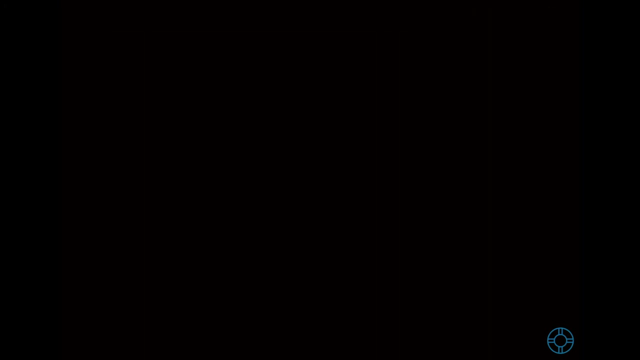 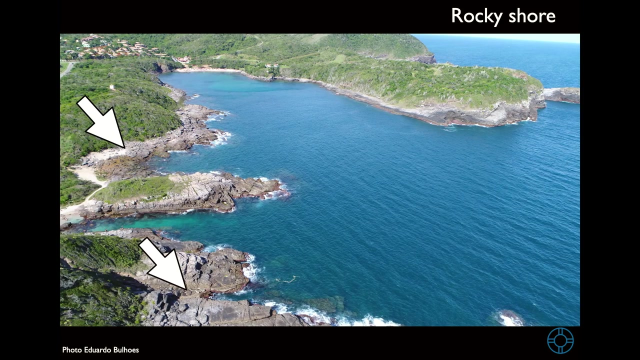 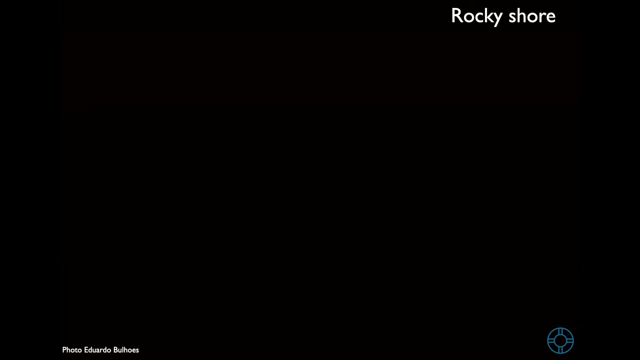 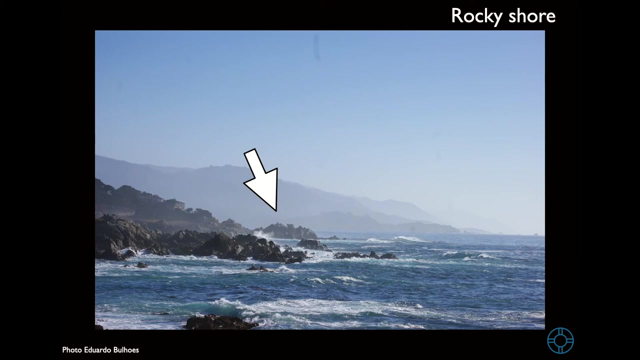 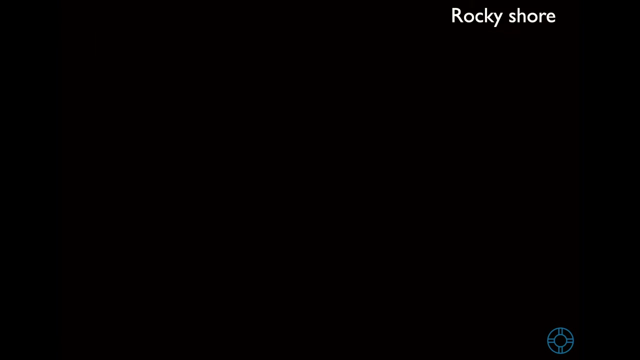 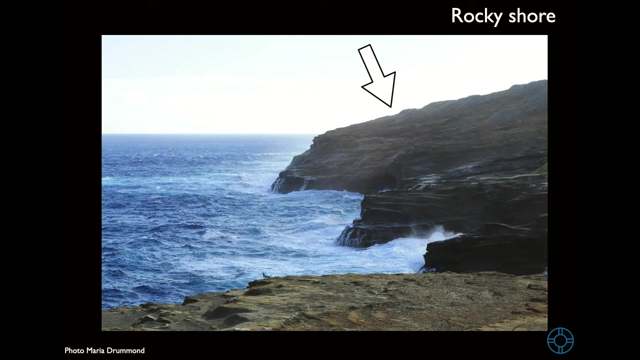 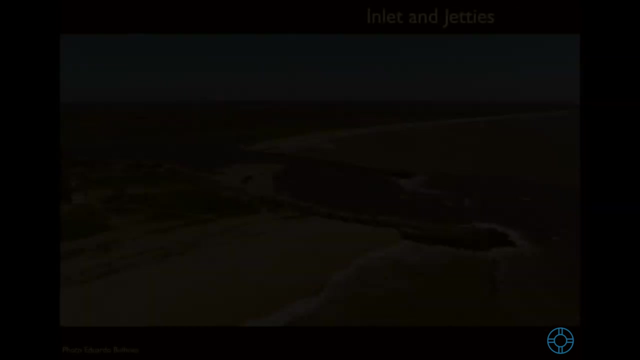 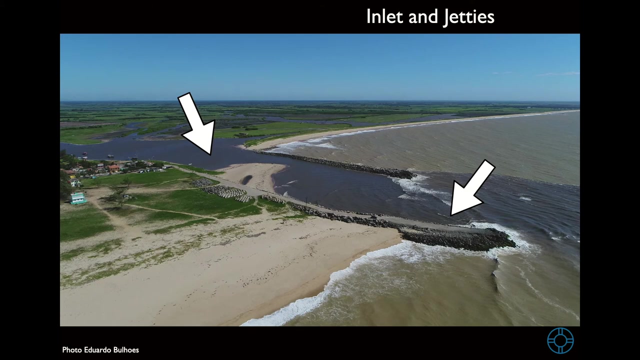 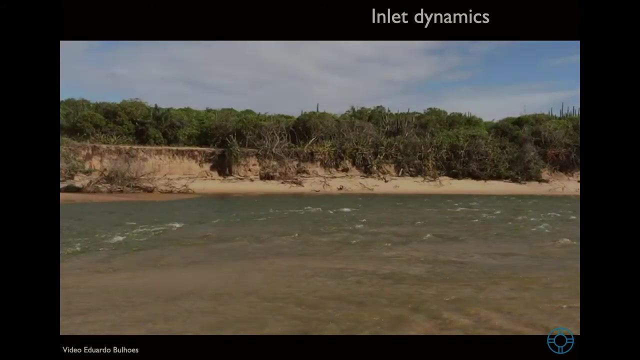 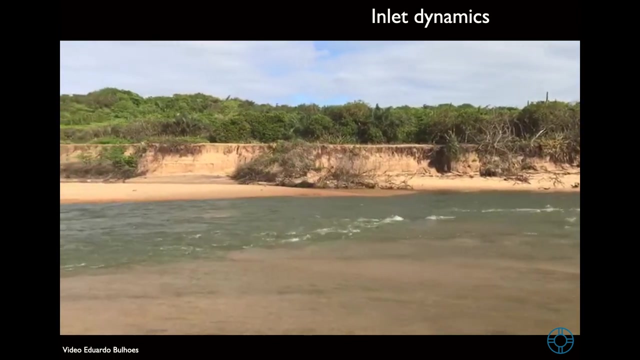 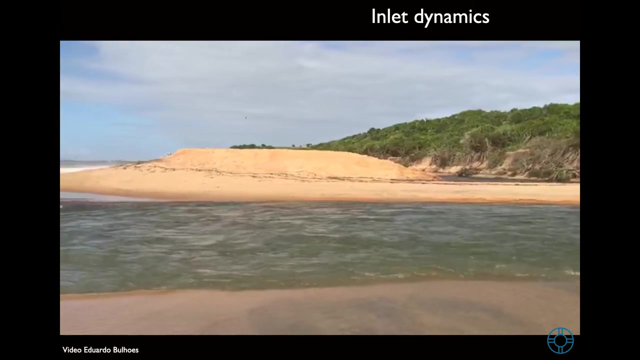 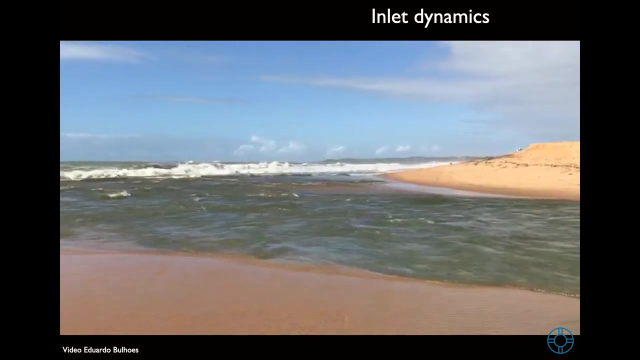 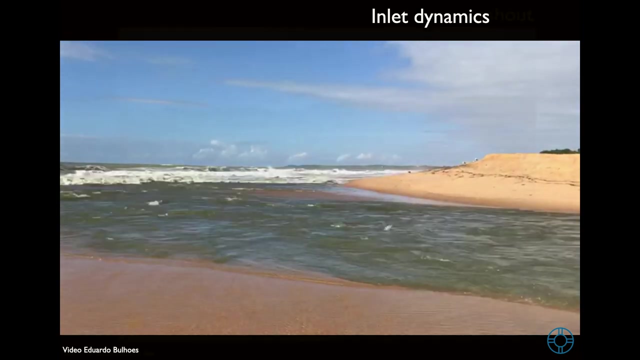 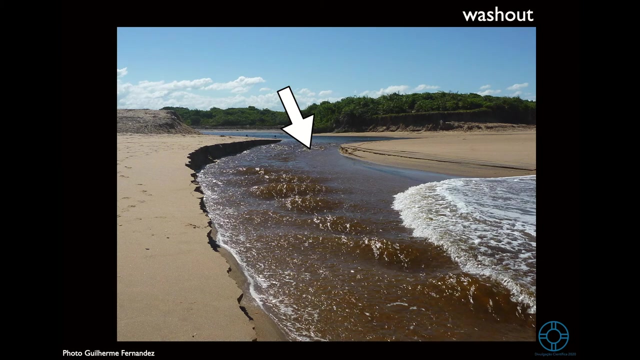 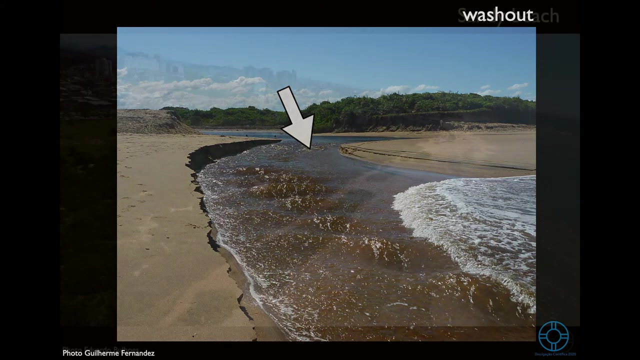 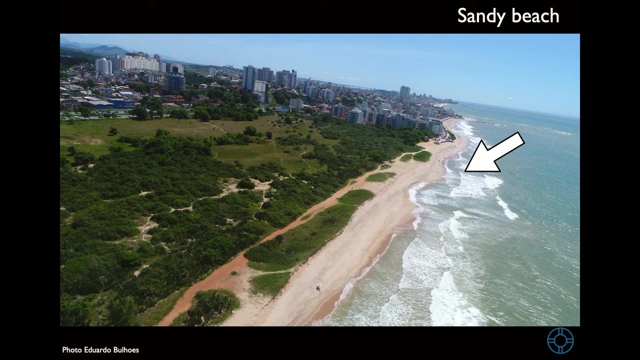 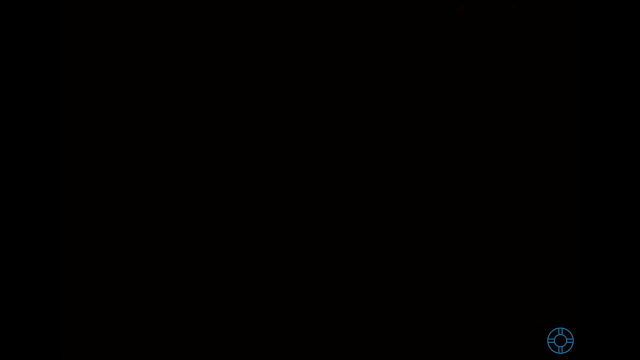 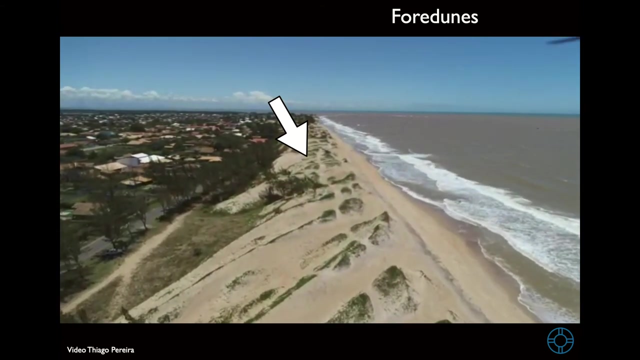 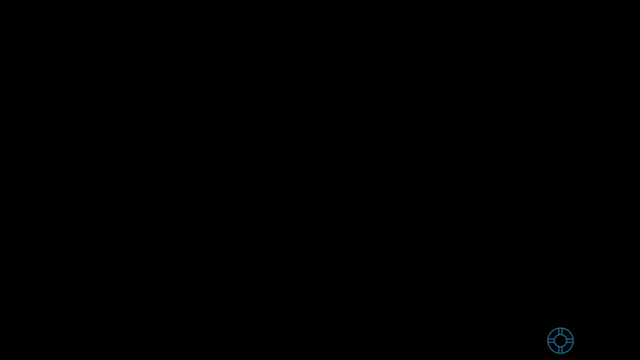 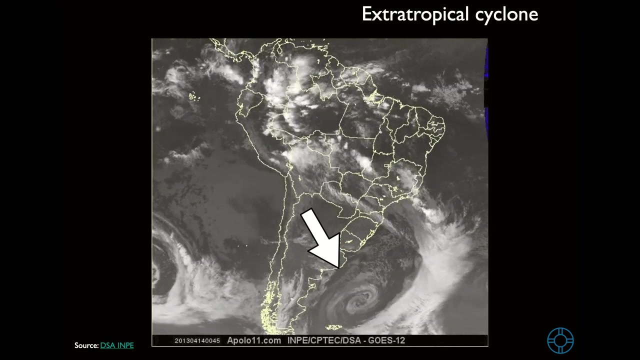 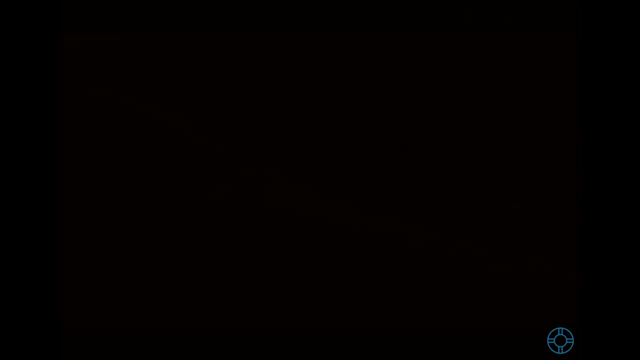 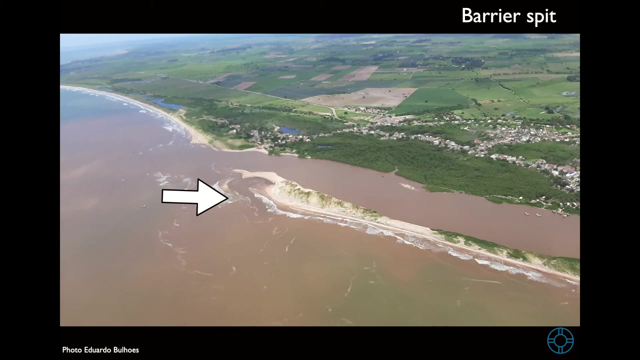 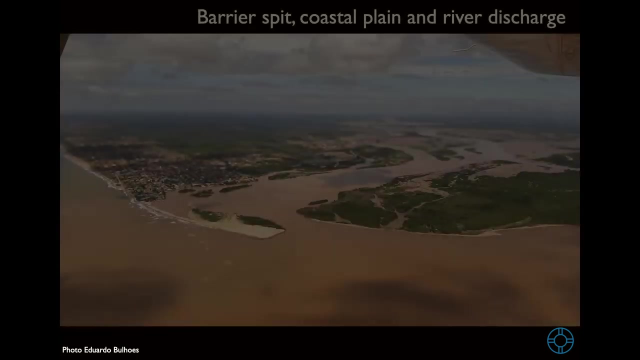 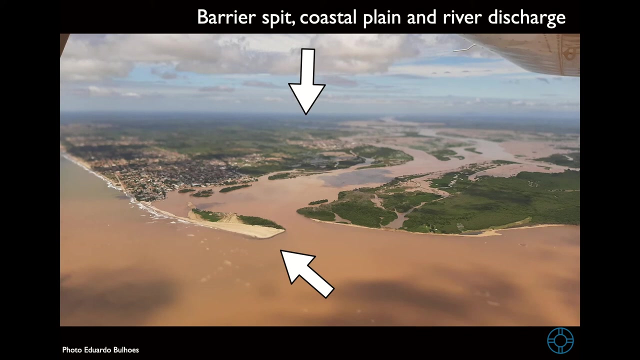 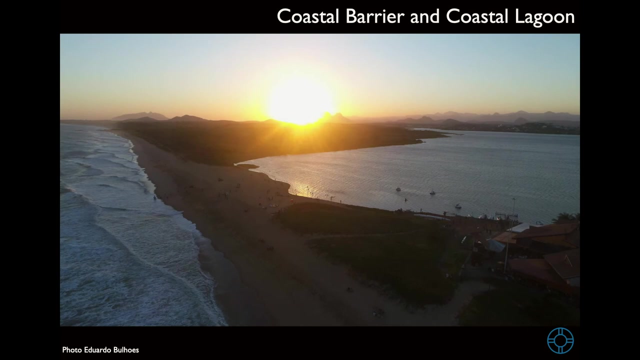 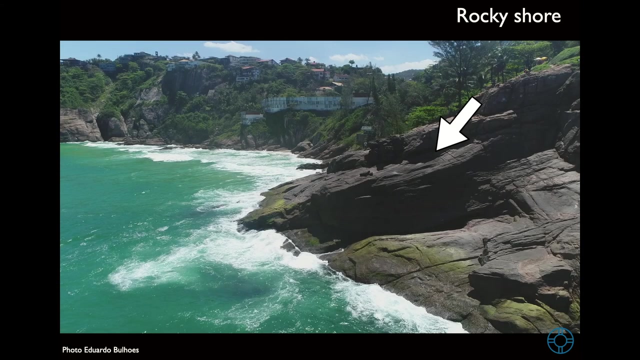 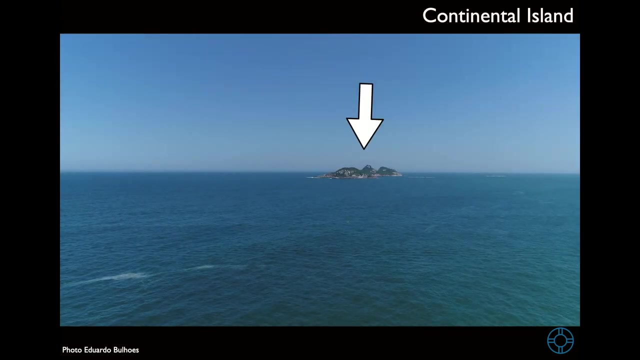 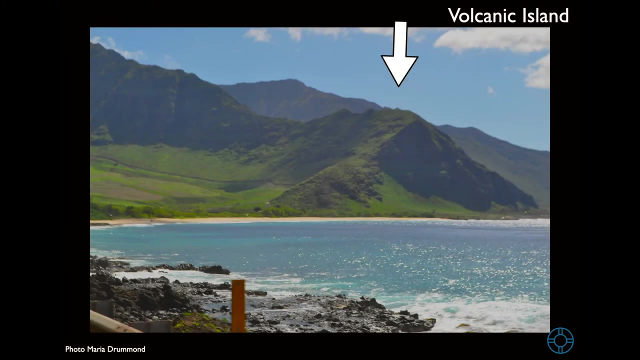 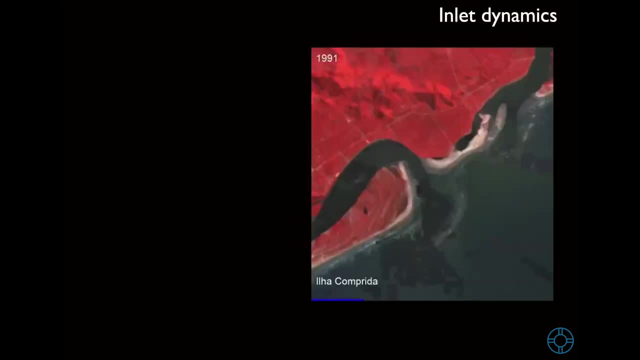 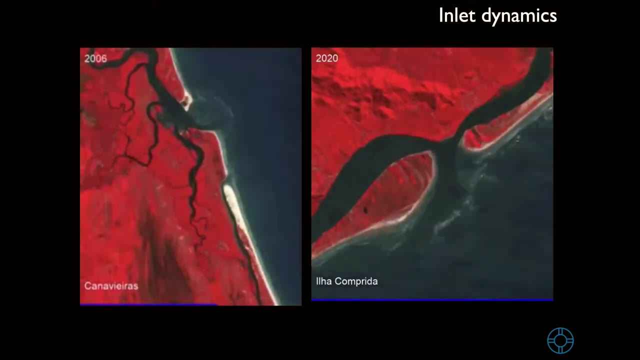 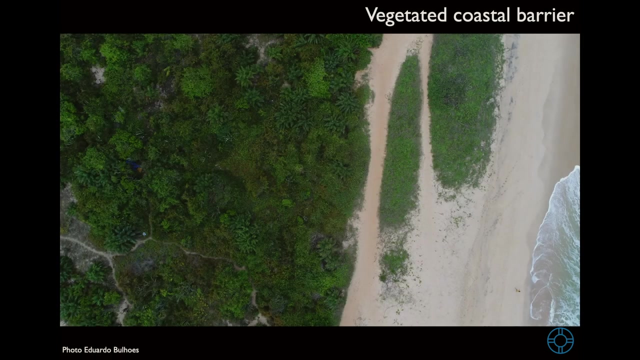 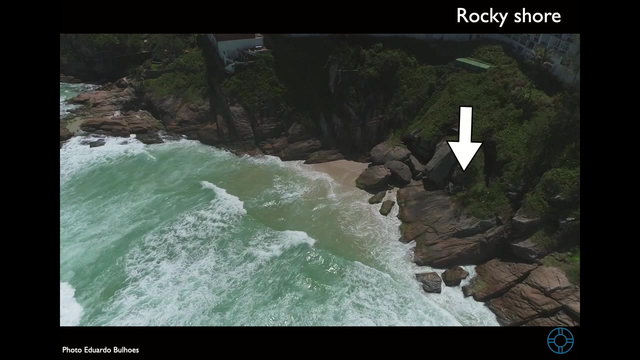 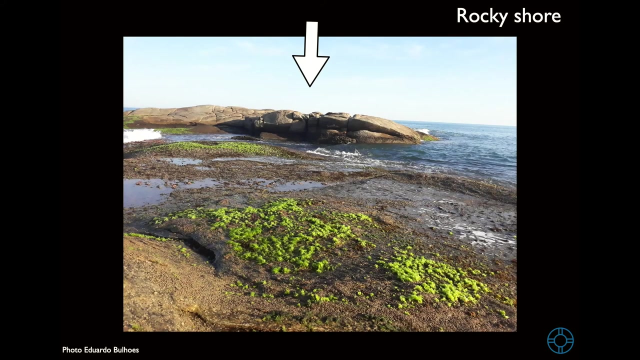 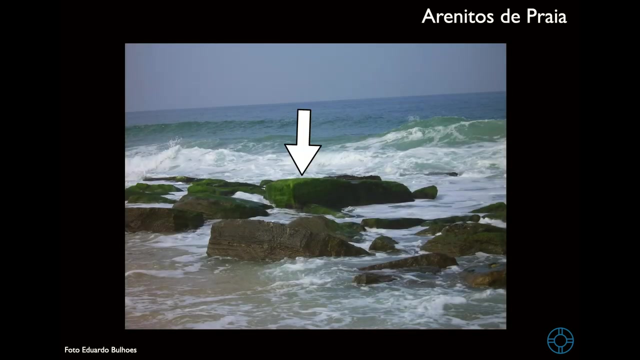 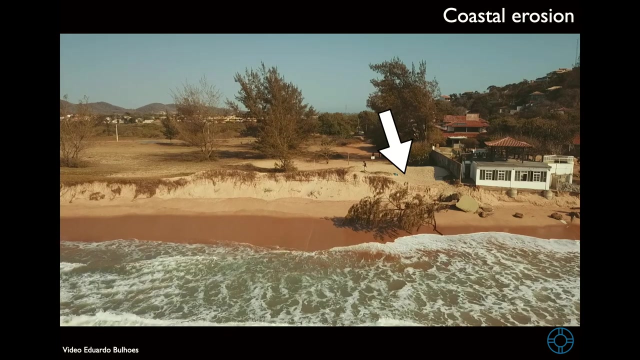 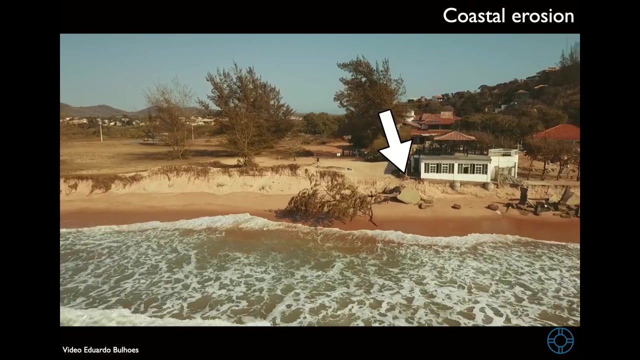 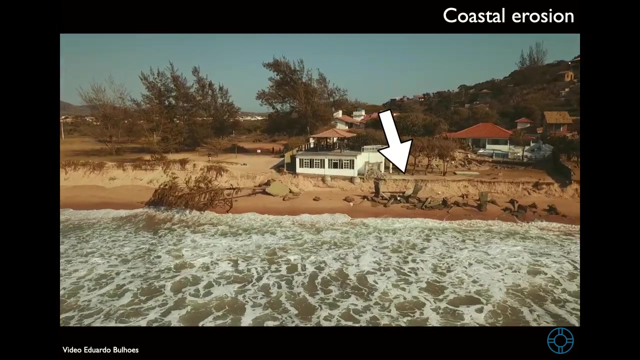 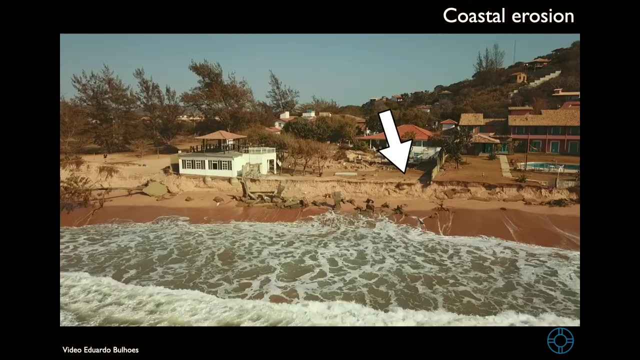 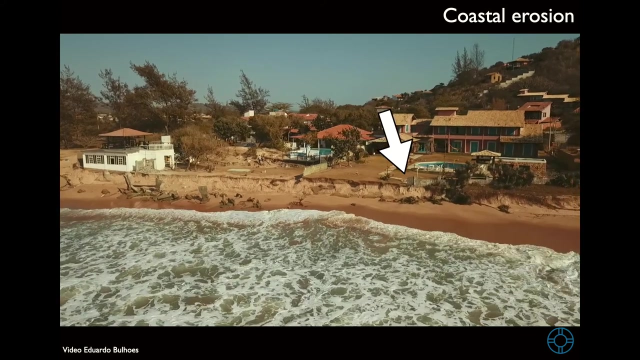 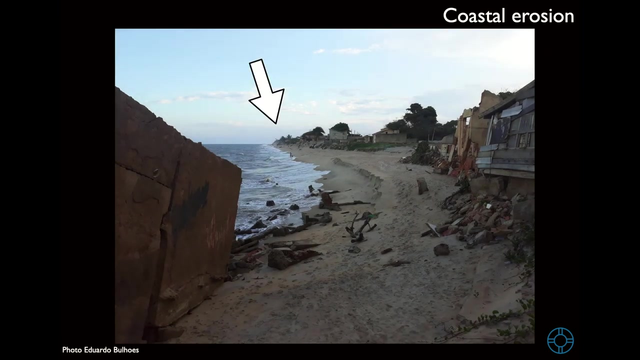 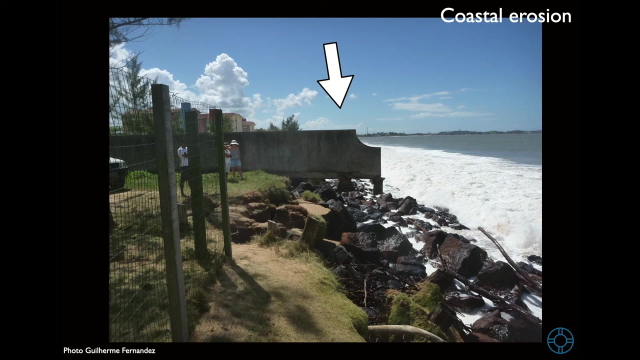 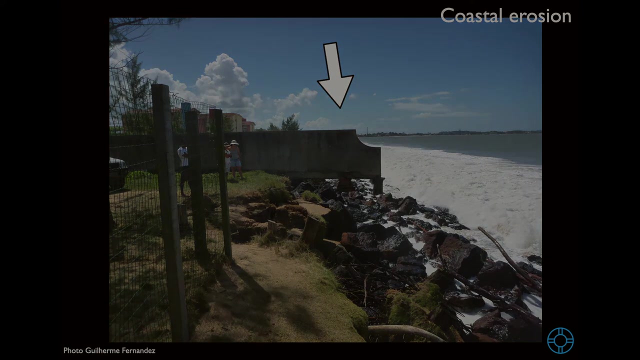 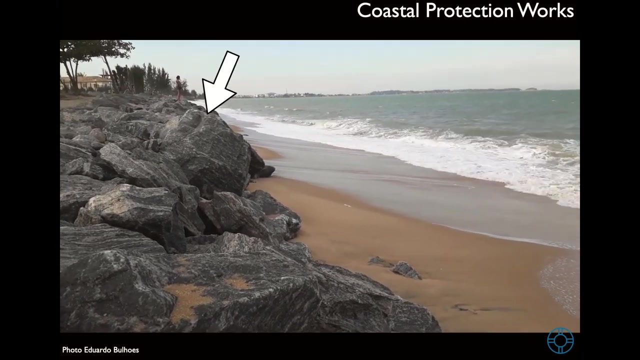 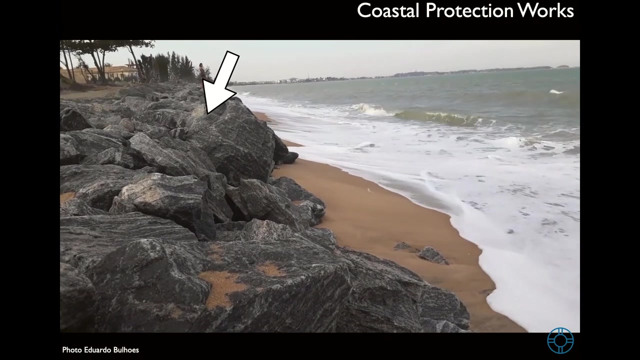 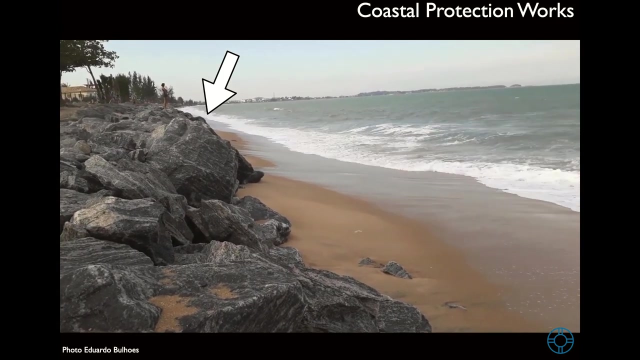 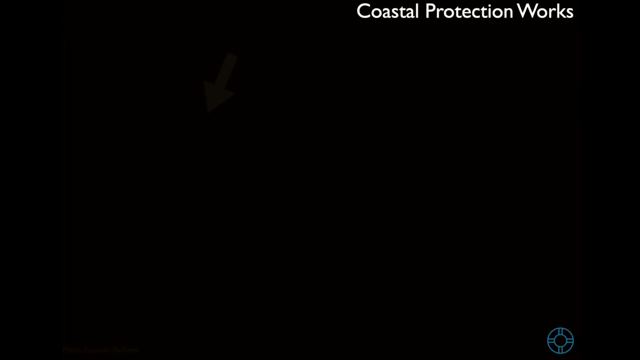 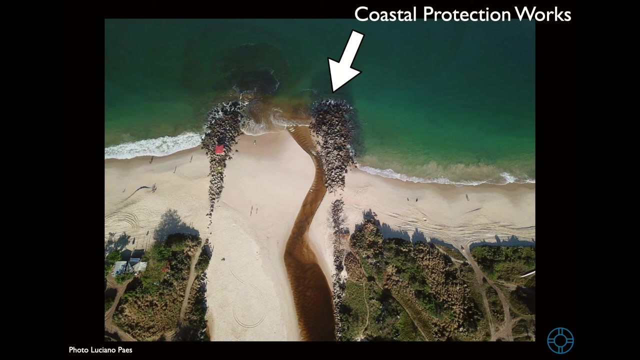 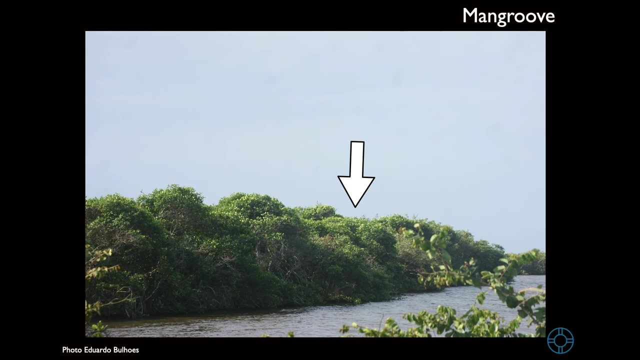 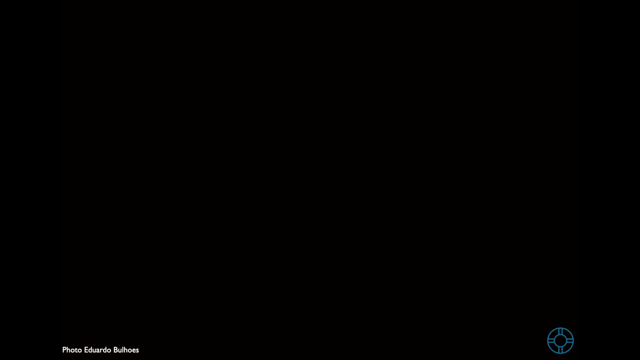 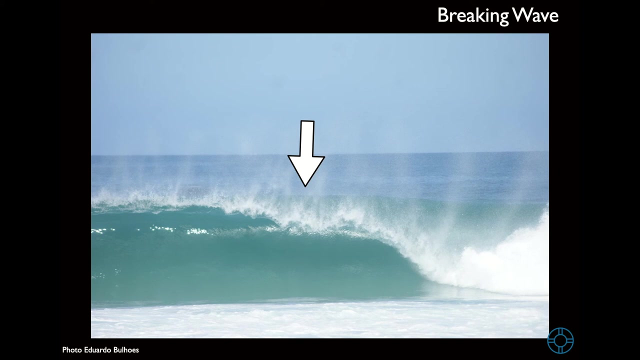 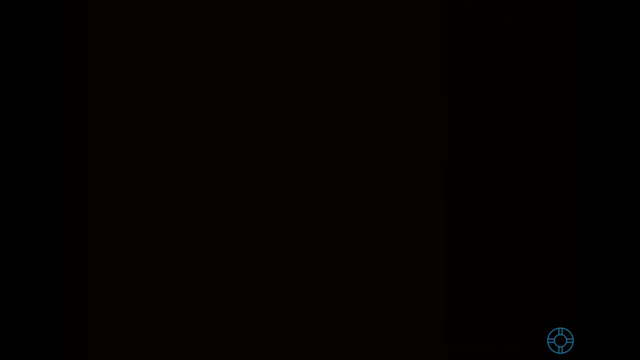 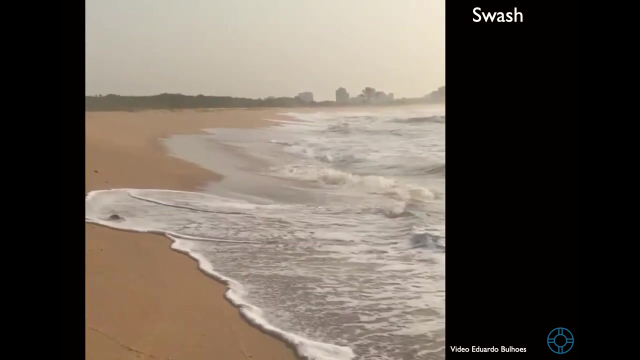 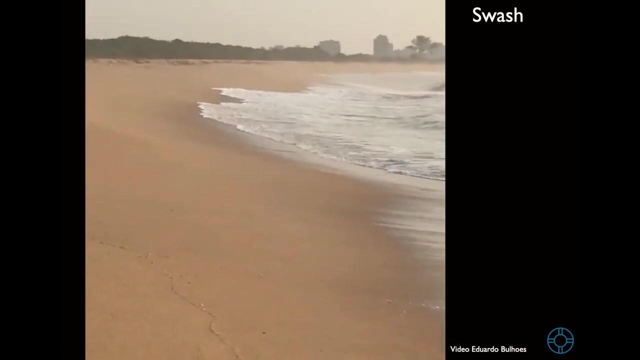 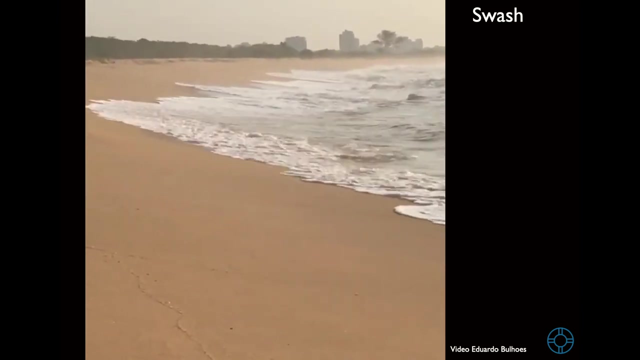 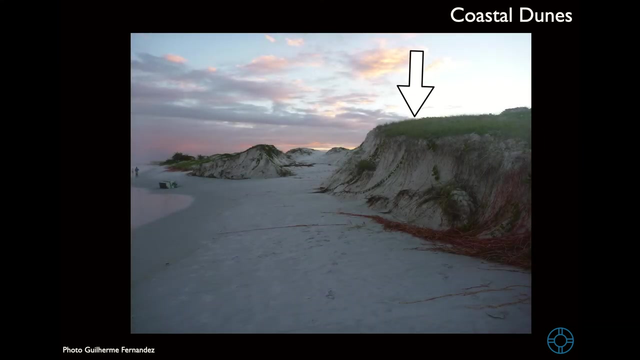 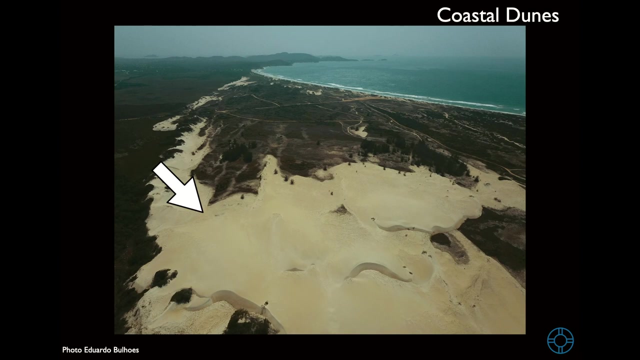 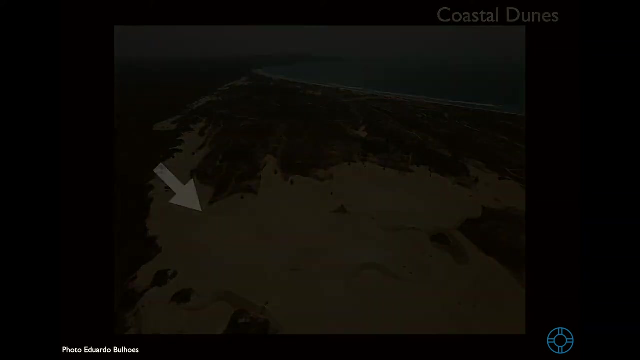 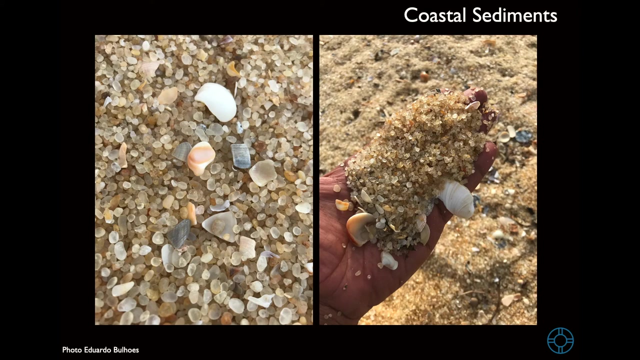 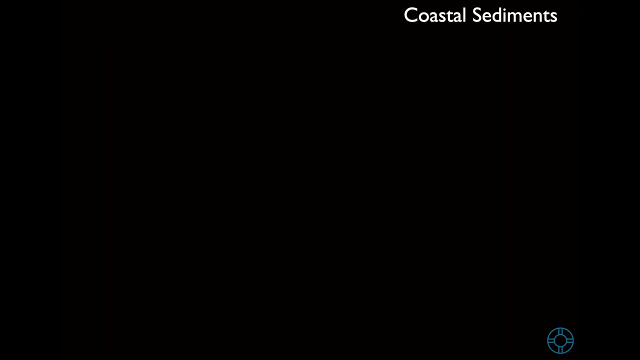 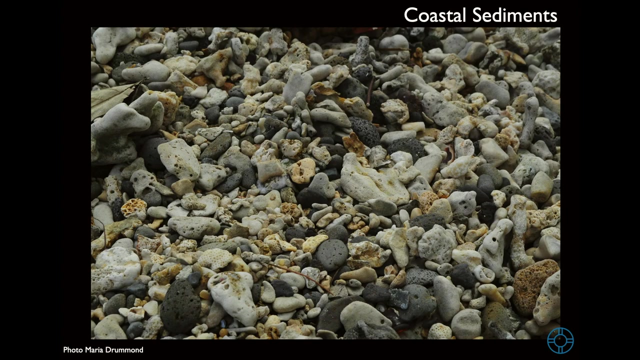 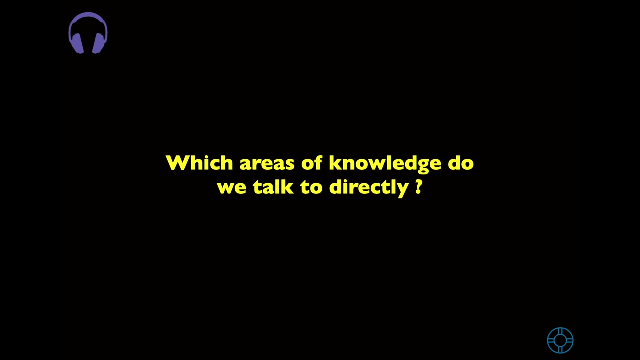